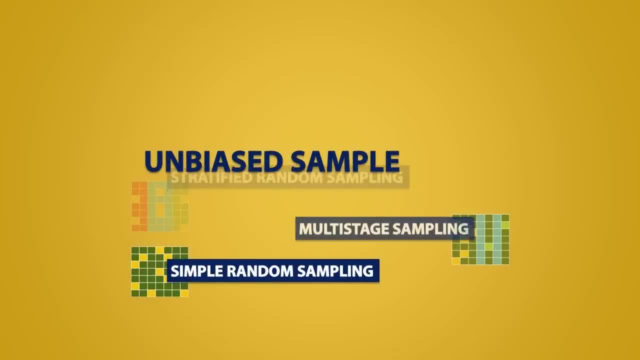 is known as an unbiased sample. We will be looking at three different types: Stratified random sampling, multistage sampling and simple random sampling. The most basic type of sampling is the simple random sample, also known as an SRS, Since. 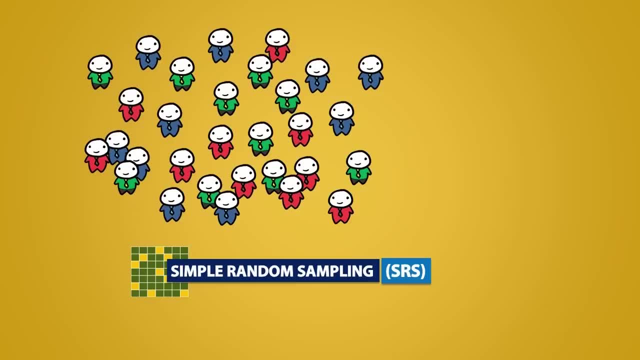 an SRS is unbiased. each individual has an equal chance of being chosen. This means that each of our figures has been selected based on how much data we have collected and what we consider the best of their kids. The emerges fraiend automic data are looked at in figure. 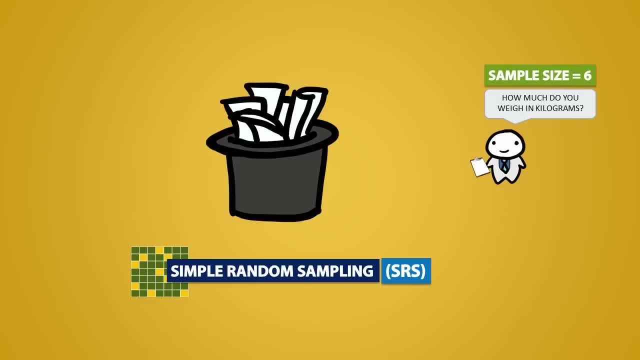 45, including the size of this cell graft, NAV and the number of cells being picked up For samples that we take actively. a sub-t assessor will take a strategy, while those urnot fazing is given such an Billie Keisler-like tip. 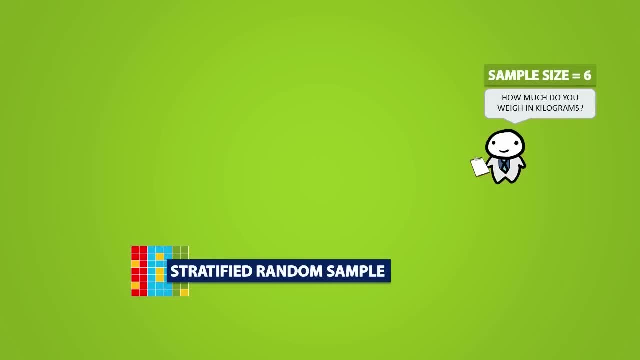 These were mother educational samples that were made FlashBotIf using Non employers. deshalb I wanted a sample size of six, in other words, to be part of the sample. You can think of an SRS as putting names into a hat and selecting n of them. So if I wanted 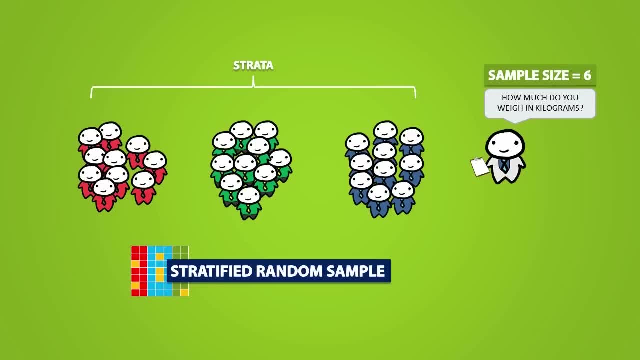 a sample size of six. I would select six papers and come up to the randomly chosen people to interview them. For a stratified random sample. we take the population and we divide it into something- an SRS- and combine the SRSs to get the full sample. For example, we could take an SRS of: 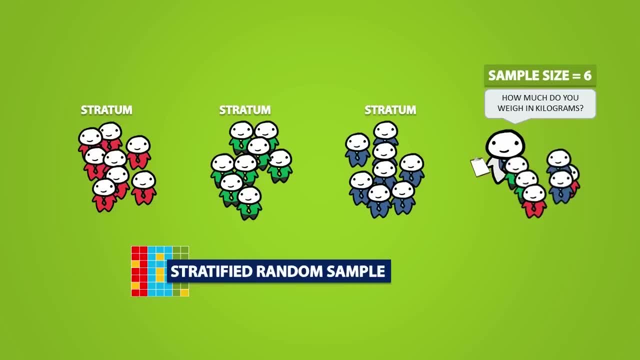 2 people from each group so that we get the total of 6 people. A stratified random sample is good for making sure that whoever is administering the sample gets in contact with each kind of group. The last type of sampling is called multistage sampling. For multistage sampling 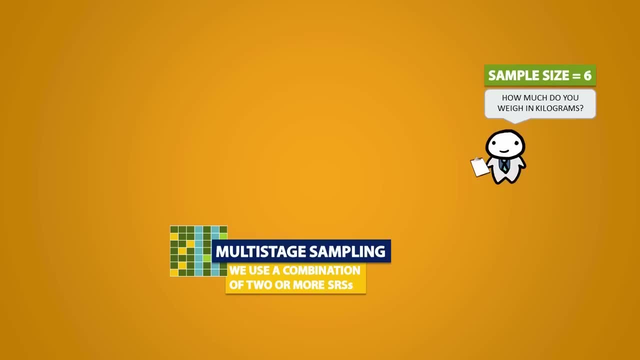 we use a combination of 2 or more simple random samples. As the name suggests, multistage sampling means you have to go through different stages to find where your sample comes from. For example, if we have 3 groups, stage 1 could be selecting which group will be picked. 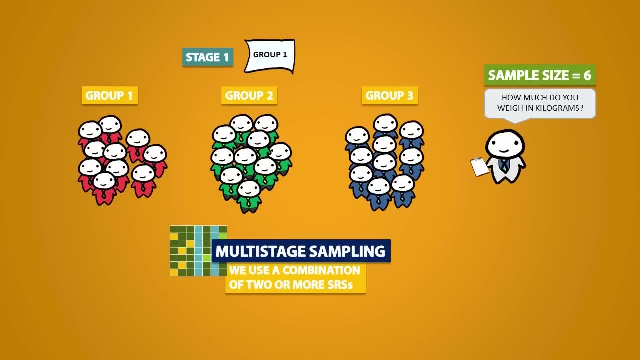 using an SRS. Let's say that I picked out group 1, then that means I would only look at group 1.. Then for stage 2, I would do another SRS to get the 6 random people. We go through different stages of simple random samples to get the actual sample, and this is why 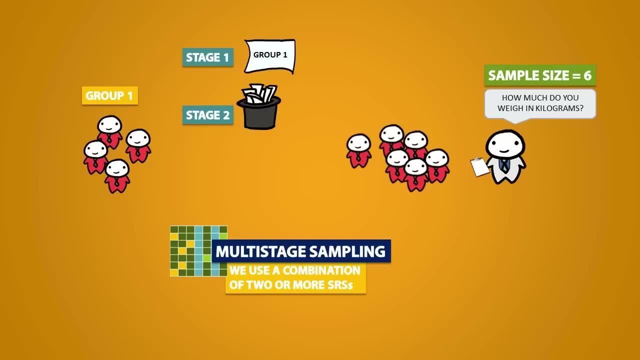 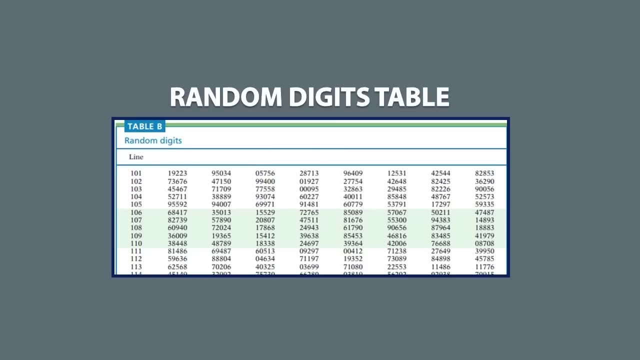 this is called multistage sampling. I'd like to point out that, instead of putting names in a hat, there's another way to pick things randomly: We can use something called the random digits table. The random digits table consists of a long string of random numbers, and it can help us do an SRS. 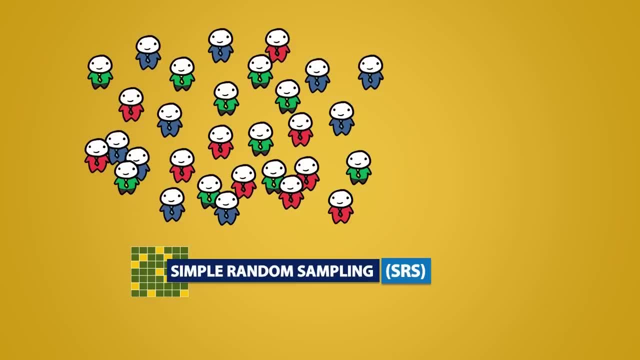 an SRS is unbiased. each individual has an equal chance of being chosen. This means that a person with random sample size of 6 would be eligible to be part of the sample. You can think of an SRS as putting names into a hat and selecting n of them. So if I wanted 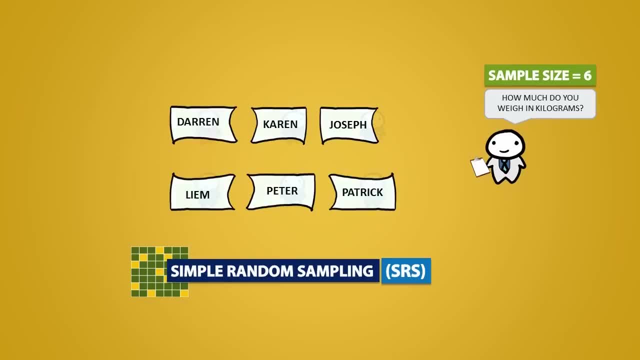 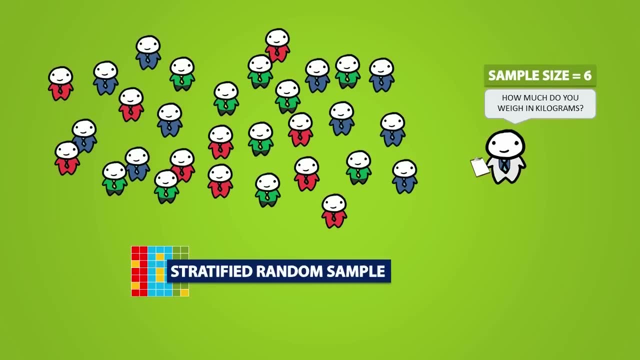 a sample size of 6, I would select 6 papers and come up to the randomly chosen people to interview them. For a stratified random sample, we take the population and we divide it into something called a strata. Strata refers to the groups of similar people Within each. 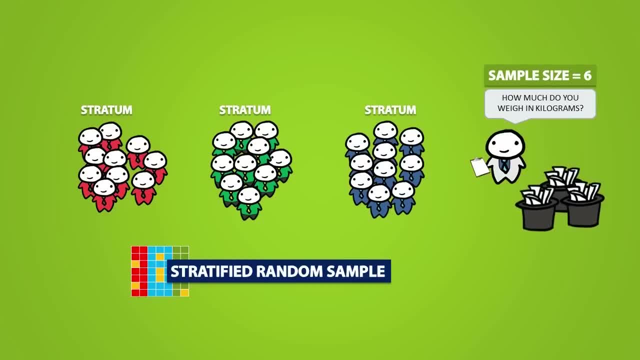 stratum. we take an SRS and divide it into 3 different groups of people- That's what we call a stratum- and combine the SRSs to get the full sample. For example, we could take an SRS of 2 people. 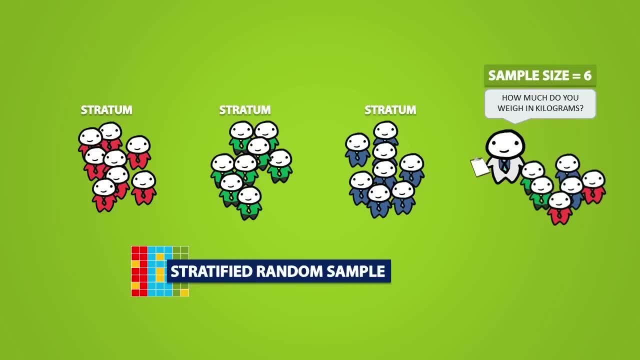 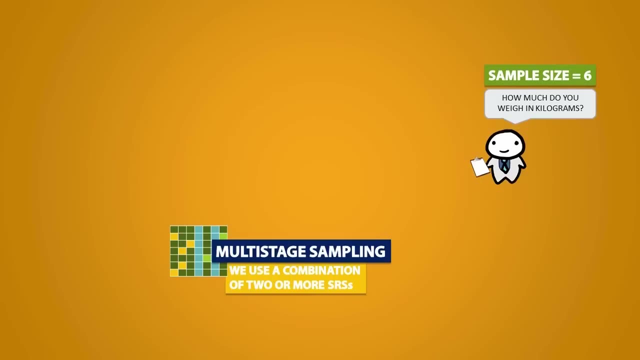 from each group so that we get the total of 6 people. A stratified random sample is good for making sure that whoever is administering the sample gets in contact with each kind of group. The last type of sampling is called multistage sampling. For multistage sampling we use a 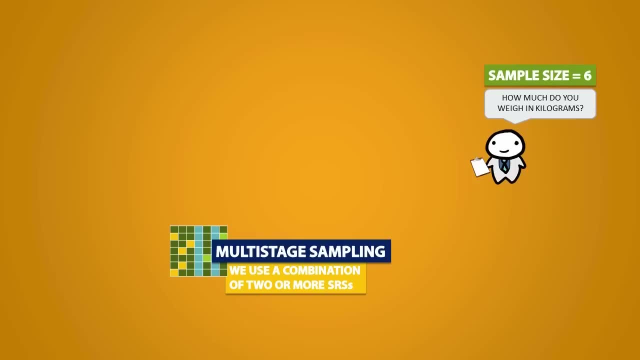 combination of two or more simple random samples. As the name suggests, multistage sampling means you have to go through different stages to find where your sample comes from. For example, if we have three sacja groups, stage 1 could be selecting which group will be picked using an SRS. 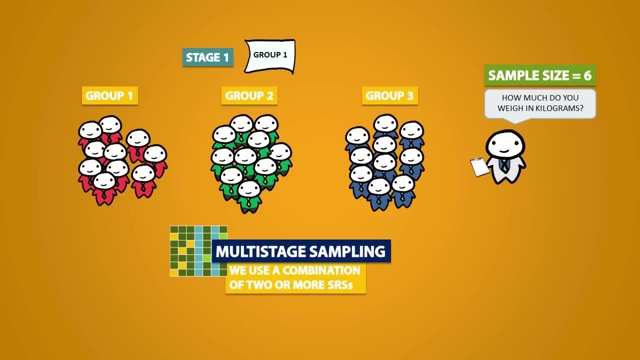 Let s say that I picked out group 1, then that means I would only look at group 1.. Then for stage 2, I would do another SRS to get the 6 random people. We go through one sample formerly of the group and look at single sample. Then in this case I just have to look at group number, simply so that it is Ideally they allistaic and the sample animal. That s all that I have And I have for stage 2, I would select one SRS to get all this, leaving at the size of 1.. 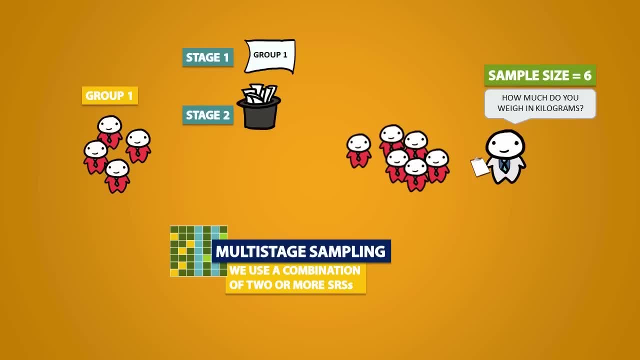 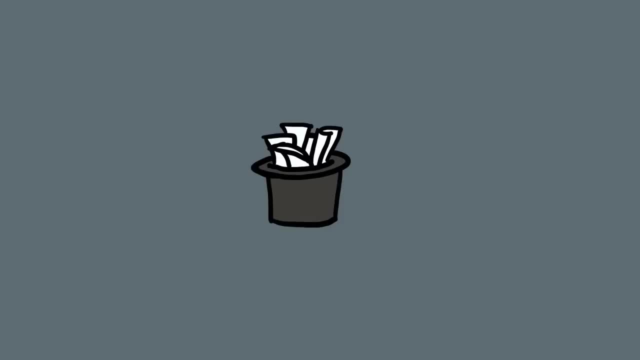 different stages of simple random samples to get the actual sample, and this is why this is called multistage sampling. I'd like to point out that, instead of putting names in a hat, there's another way to pick things randomly: We can use something called. 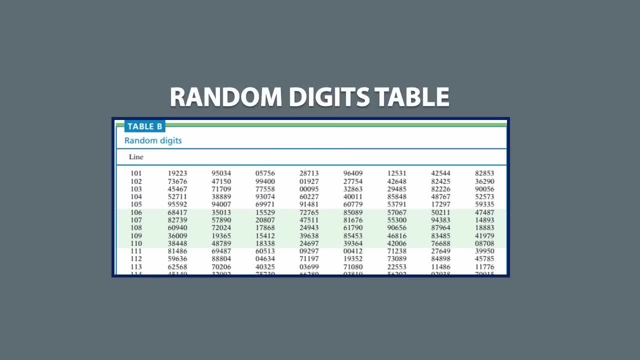 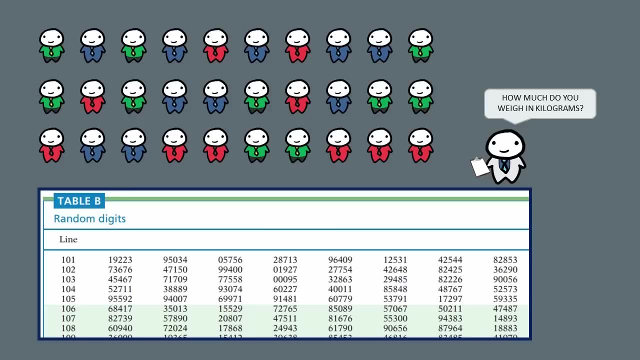 the random digits table. The random digits table consists of a long string of random numbers and it can help us do an SRS. To use it, I would first have to label each member of the population with a number. We have 30 people in this population, so I will label. 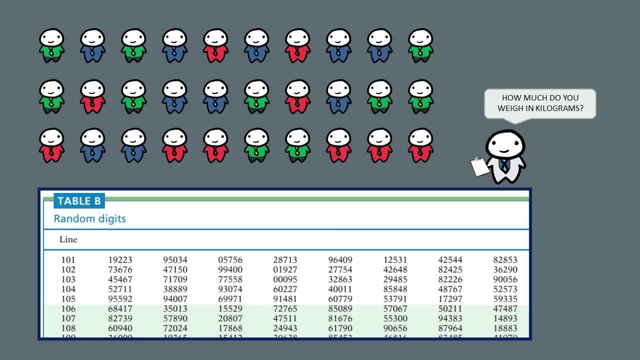 To use it, I would first have to label each member of the population with a number. We have 30 people in this population, So I will label each person from 1 to 30.. Notice how I have written 01 instead of just 1.. 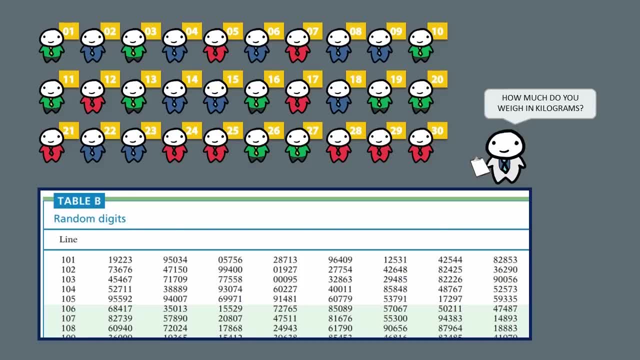 Doing this helps us use the random digits table. Since each label has two digits, we will read the string of numbers, two digits at a time. So let's say I want a sample size of 4.. We will use the random digits table to randomly select 4 people. 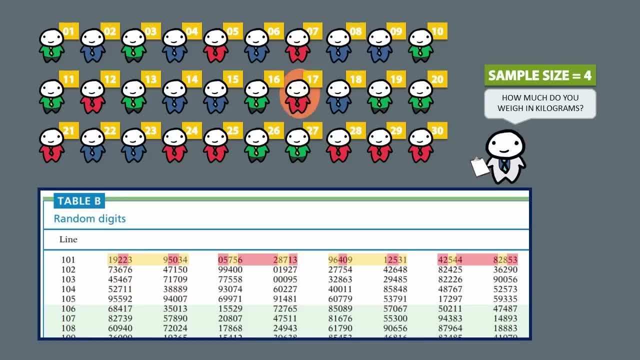 The first number on the table is 19,. so person 19 will be part of the sample. The second number is 22.. So person 22 will be part of the sample. The third number is 39, but our sample size doesn't go. 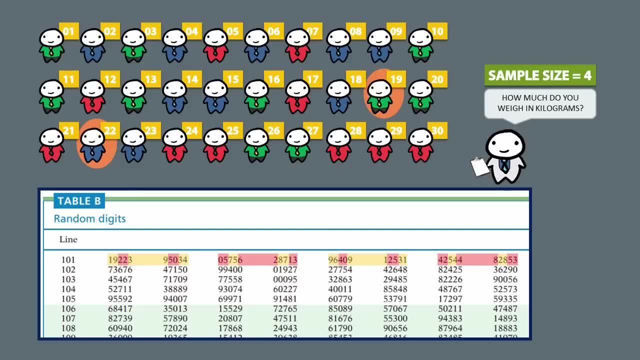 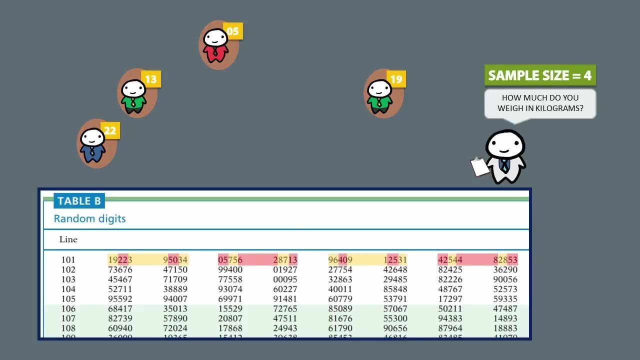 up to 39,, so we will ignore it. We will also ignore 50 and 34,, but we will keep number 5.. We will also ignore 75,, 62, and 87,, but we will keep number 13.. As a result, these are the people we would survey. 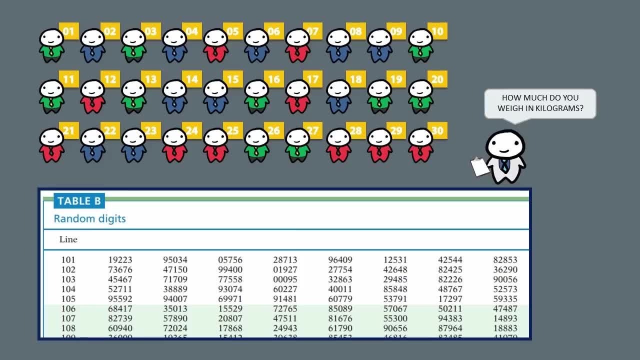 each person from 1 to 30. Notice how I have written 01 instead of just 1.. Doing this helps us use the random digits table. Since each label has 2 digits, we will read the string of numbers, 2 digits at a time. So let's say I want a sample size of 4.. We will use the 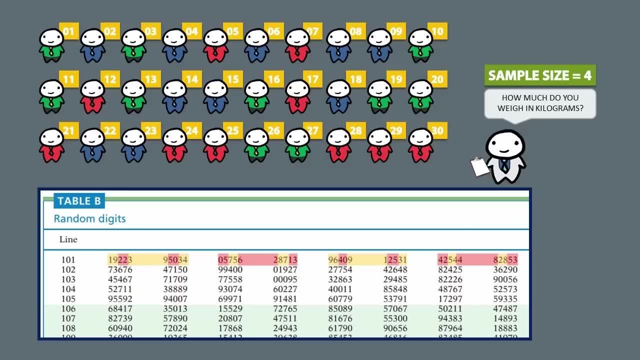 random digits table to randomly select 4 people. The first number on the table is 19,. so, put, person 19 will be part of the sample. The second number is 22,. so person 22 will be part of the sample. The third number is 39, but our sample size doesn't go up to 39, so 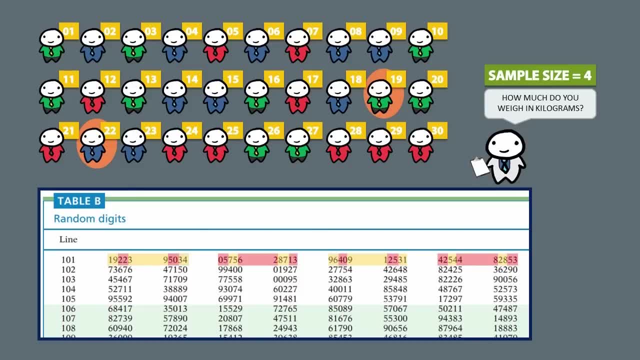 we will ignore it. We will also ignore 50 and 34,, but we will keep number 5.. We will also ignore 75,, 62, and 87,, but we will keep number 13.. As a result, these are the people. 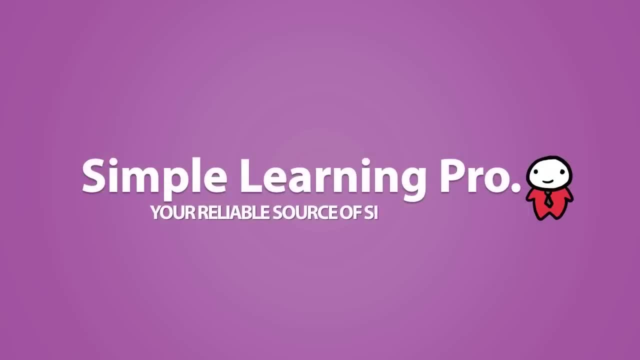 we would survey Subtitles by the Amaraorg community. 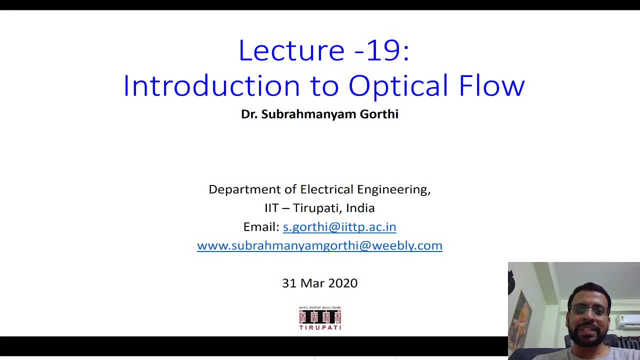 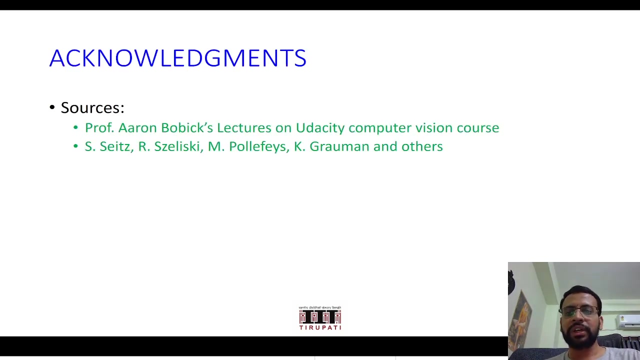 Hi students, welcome to the second online video lecture of computer vision. This is on introduction to optical flow. Hope you have gone through the previous lecture on introduction to motion estimation. This is a continuation of that. Okay, let's go ahead. Like the previous video lecture, this has been also an adaptation of the content. A lot of content has been adopted from Professor Arun Bobik's lecture on introduction to computer vision, on Adacity, and some slides from other sources. 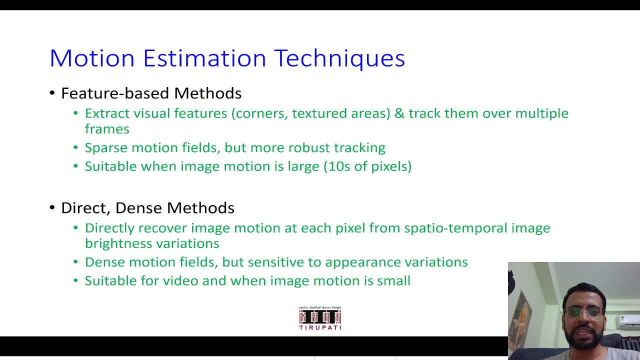 This is a recap slide from the previous lecture. The motion estimation techniques can be divided broadly into two categories. One is the feature-based methods and another is the direct-dense-based methods. Feature-based method is in a given image and its subsequent frame you would be capturing.